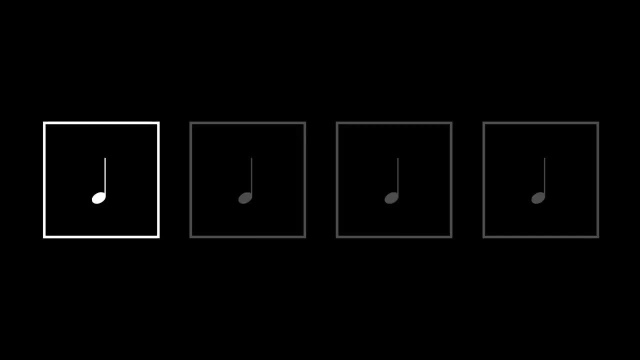 clapping along with the beat. This way, you're sure to always be feeling the beat in your body, And we're going to vocalize all the rhythms. So let's start with the quarter note beat itself: Da da, da da. 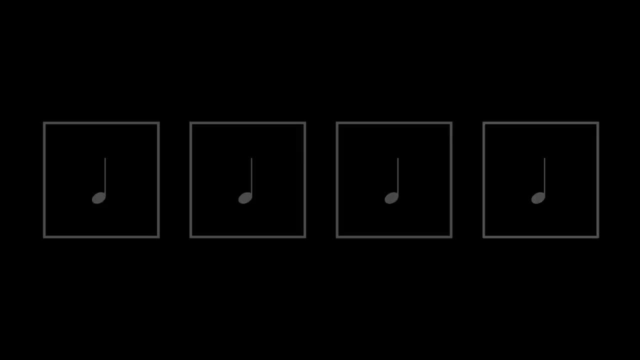 And we're using the syllable, by the way, because it has a percussive, clearly defined attack And we're just trying to memorize the abstracted feeling of each rhythmic figure. So changing numbers or syllables, as is common in rhythmic counting, is actually not very helpful for this. 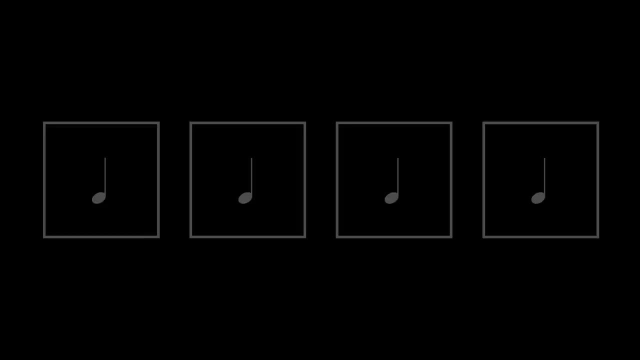 and can be a bit of a distraction. Also, don't worry about sustaining. Think of the sound you're making as a drum hit. Okay, you try it. Keep tapping your foot or clapping and vocalize on each beat. Easy enough, Now let's subdivide the beat into two equal parts. Recall these. 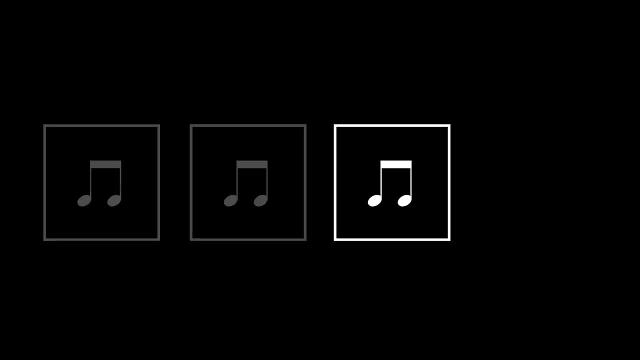 eighth notes: Da da, da, da, da, da da. Now you try it, vocalizing eighth notes while also tapping or clapping the quarter note beat. Here we go, Here we go Now. be careful that you didn't change your clapping or tapping of the beat. 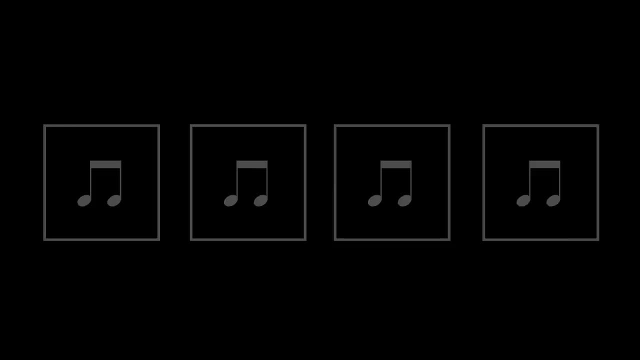 to match what you were counting. You keep tapping even quarter notes and you vocalize the rhythm itself. Okay, let's keep going. If we subdivide the eighth notes in half, we get sixteenth notes, the beat divided into four even pieces. 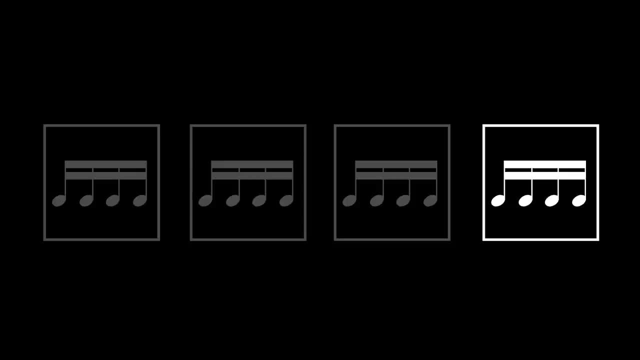 Dun-dun-dun-dun-dun-dun-dun-dun-dun-dun-dun-dun-dun-dun-dun-dun. You might notice that I'm emphasizing the syllables that occur on the beat. This is important. 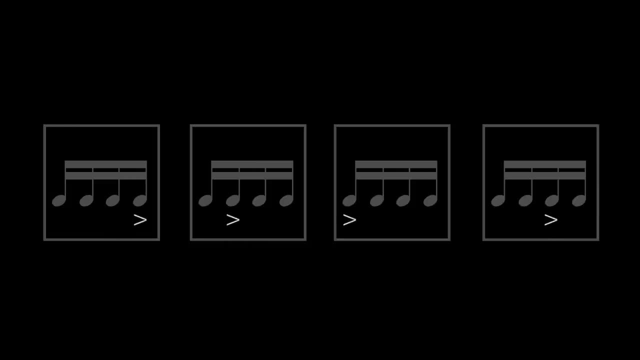 Where the emphasis falls changes our perception of the figure itself, even if it's using the same note values. Okay, your turn. So you have to vocalize a lot of syllables there, but keep yourself anchored, thinking about evenly spacing the four sixteenths across the beat. 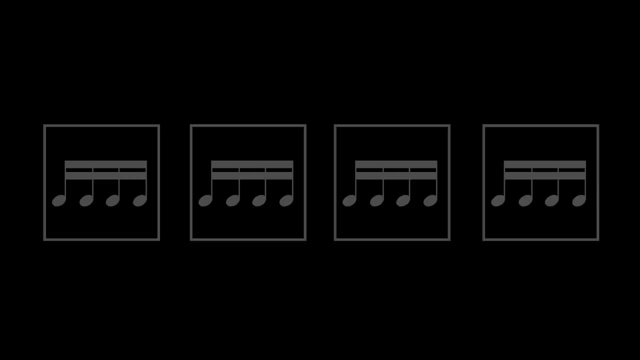 If you find you're having trouble staying locked in with the beat that you sort of drift away from it, don't worry, That's not uncommon at first, But keep at it. This is a skill that gets better with practice And when you're recording in the studio. 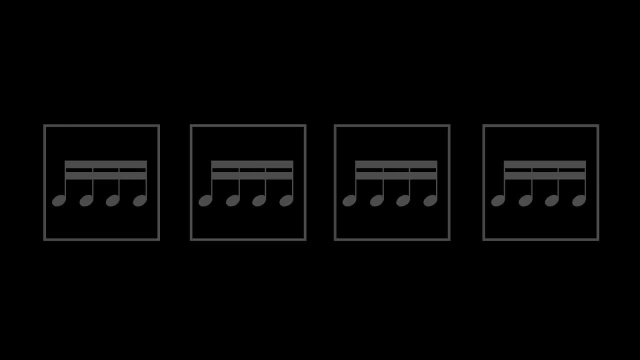 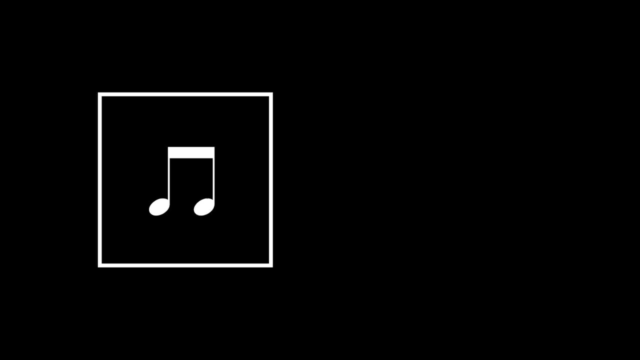 or performing with other musicians. remaining steady with the beat is just non-negotiable. You have to be able to do it All right. moving on, We can mix and match eighth notes and sixteenths to fill out one beat three different ways. 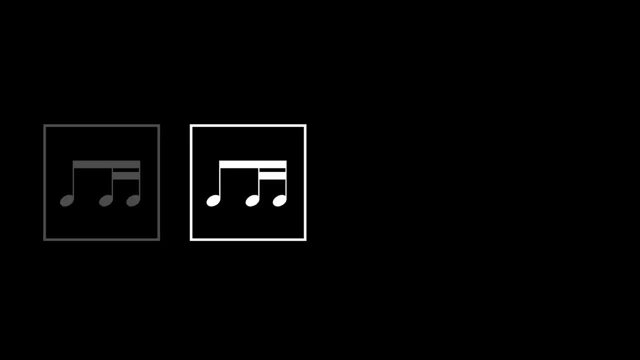 Eighth and two sixteenths. Dun-dun-dun-dun-dun-dun-dun-dun-dun-dun-dun-dun-dun-dun, You go, We can do two sixteenths and an eighth. 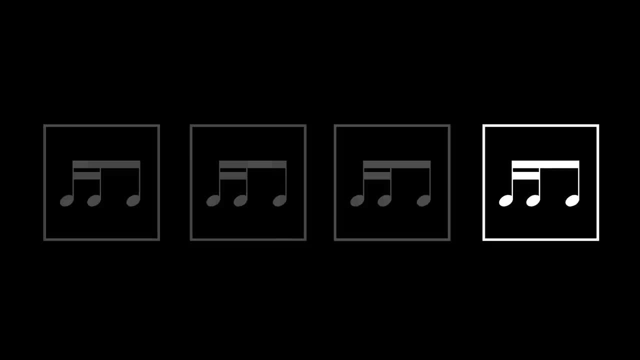 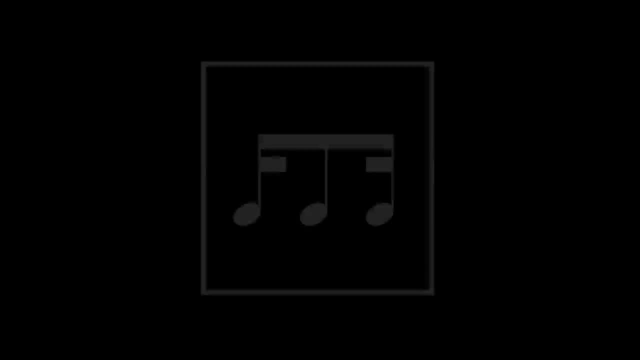 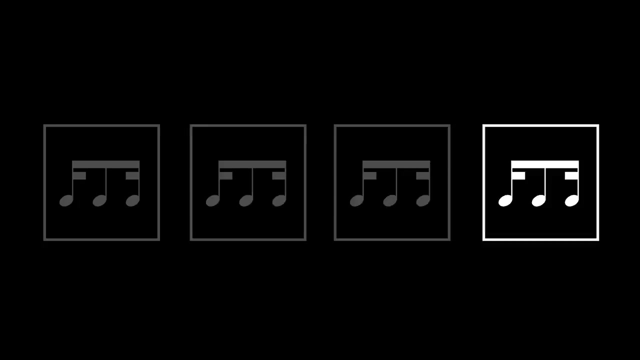 Dun-dun-dun-dun-dun-dun-dun-dun-dun-dun-dun-dun-dun-dun, Give that a go And a sixteenth, eighth, sixteenth, Dun-dun-dun-dun-dun-dun-dun-dun-dun-dun-dun-dun-dun-dun. 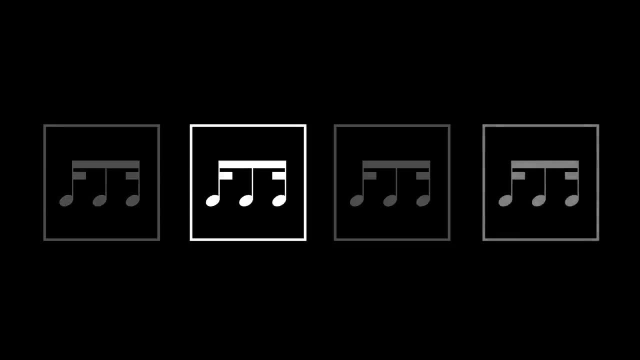 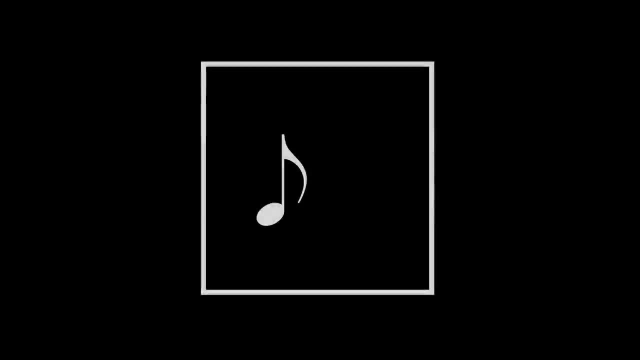 Now get this one going. Great. Now we're going to do a couple dotted eighth note figures. Eighth notes take up 50% of the beat and when you add a dot they take up 75%. To make a one beat figure with this, we add a sixteenth note. 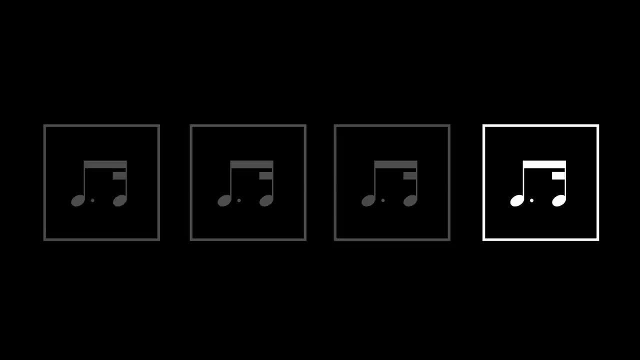 Dun-dun-dun-dun-dun-dun-dun-dun-dun. And you try it, And of course we can turn this around, so it's sixteenth dotted eighth, Dun-dun-dun-dun-dun-dun-dun-dun-dun-dun-dun-dun. 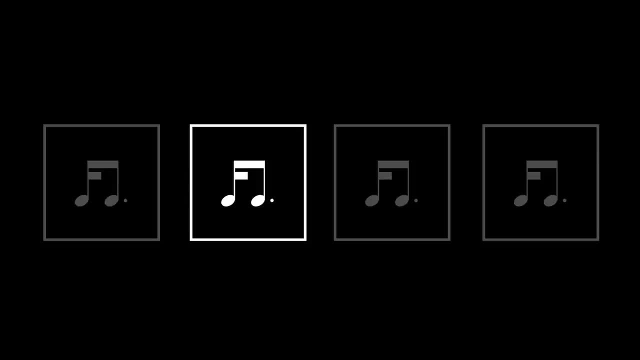 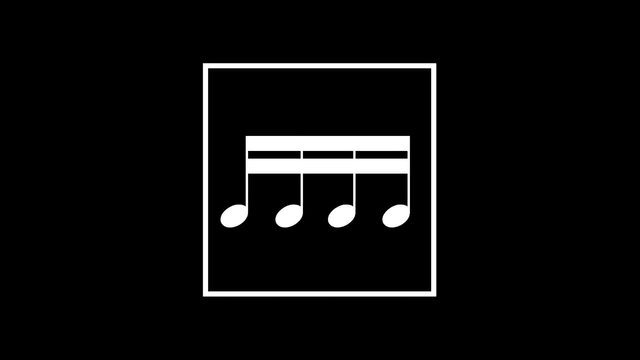 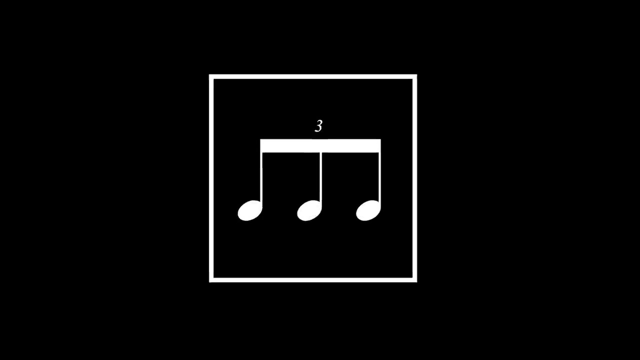 And you give it a go Now. all of these resolve down to a basic subdivision of the beat in twos or fours. but that's not the only way we can subdivide the beat. Let's subdivide it in threes. This gives us triplets. 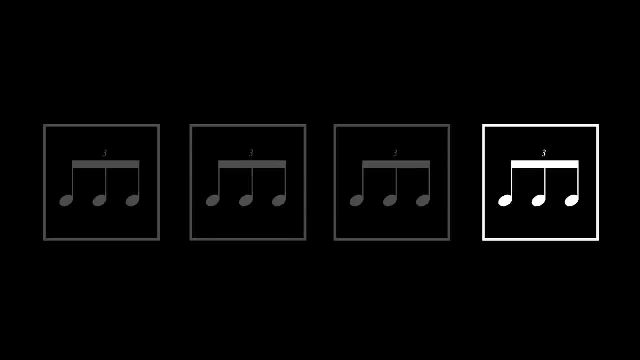 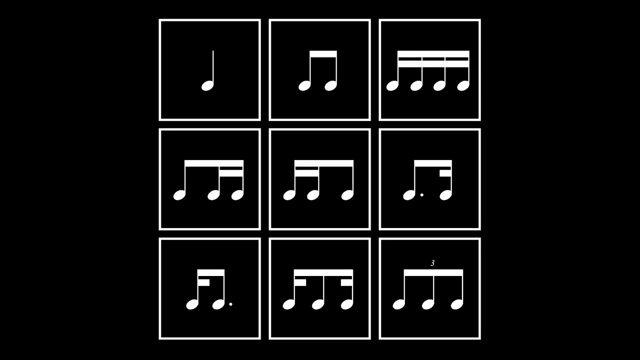 Dun-dun-dun-dun-dun-dun-dun-dun-dun-dun-dun-dun-dun-dun. Spacing out three notes evenly within one beat, Here we go. Nice, Now you just performed the nine most common one beat rhythmic figures that exist. 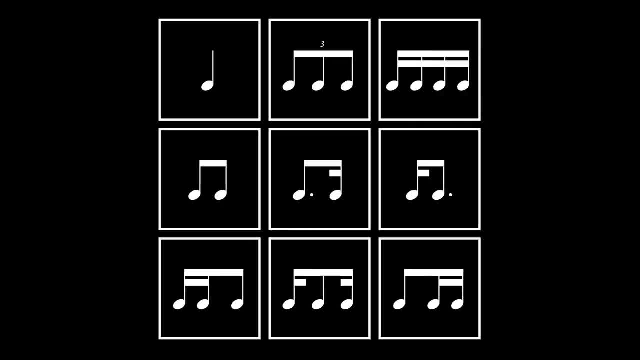 In fact, simply by arranging these nine figures in the right order and with the appropriate use of rests, you'll be able to perform a staggering number of guitar strumming patterns, piano, bass, drum, grooves, vocal melody, rhythms, the works. 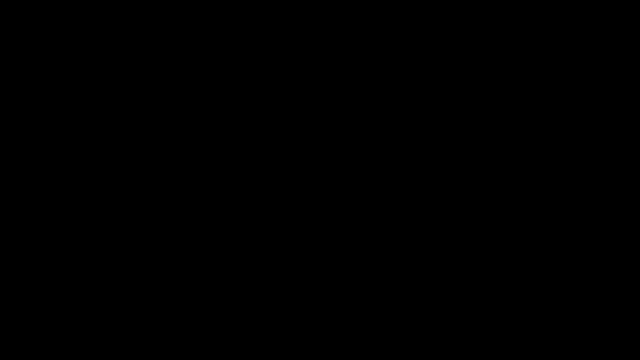 So let's do a quick roundup of all the figures we learned. Repeat them after me: Dun-dun-dun-dun-dun-dun-dun-dun-dun-dun-dun-dun-dun-dun-dun-dun-dun-dun-dun. 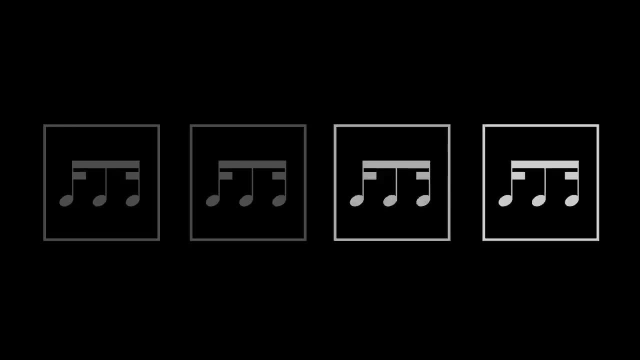 Dun-dun-dun-dun-dun-dun-dun-dun-dun-dun-dun-dun-dun-dun-dun-dun-dun-dun-dun-dun-dun-dun-dun-dun-dun-dun-dun. 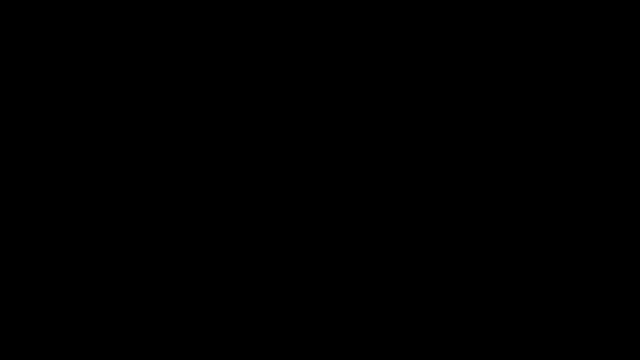 Great. Okay, now that you've got all of these figures in your ear, let's play a game. The rhythm machine is going to generate a four-figure pattern for us. Okay, there, it is Perfect one to start on. think back to how each of those sounded. now do it, and here's. 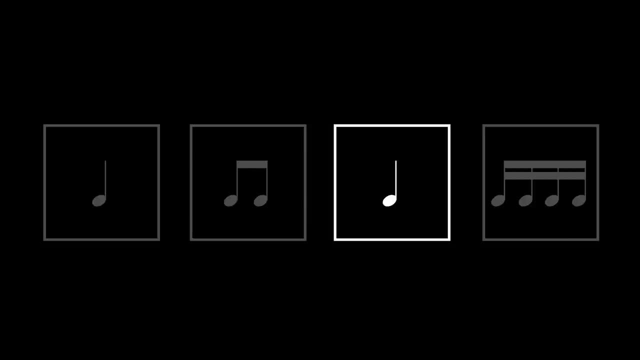